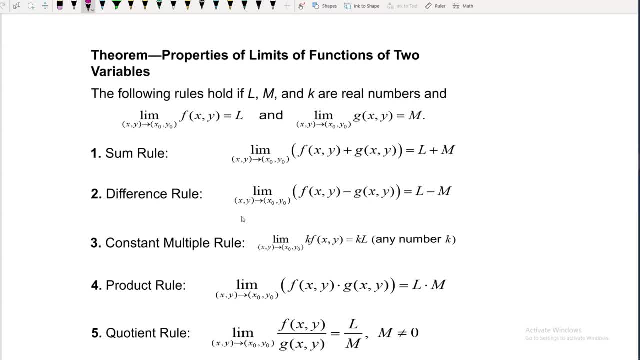 The following rules hold: if l, m and k, m and k are real numbers and limit as x and y approaches x0, y0 of f of x- y equal to n And limit as x- y approaches x0, y0 of g of x- y equal to n. 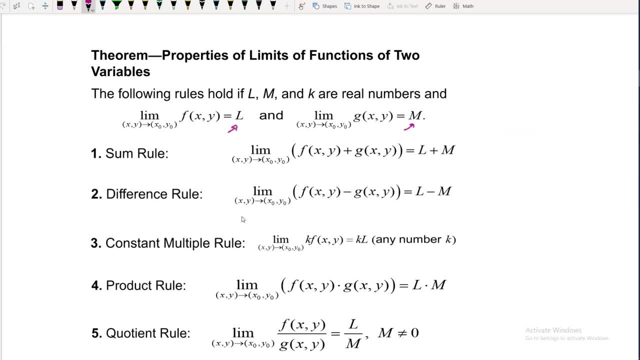 Number one: sum rule. Here we have limit as x y approaches x0, y0 of f of x- y plus g of x- y. So here we have plus. We're going to use what we had on this part and add here. 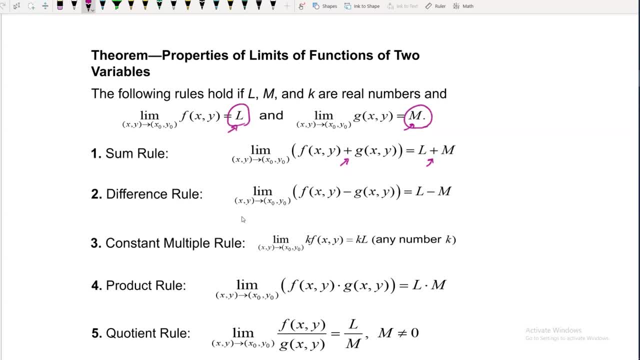 So we have l plus m, Now difference rule. We're going to have exactly the same as what we did on number one, but instead of addition we have subtraction. So limit as x, y approaches x0, y0 of f of x. 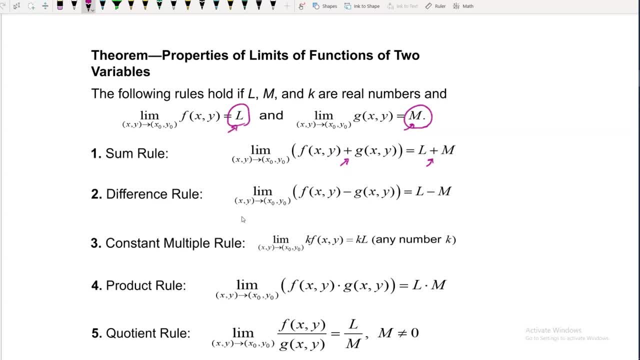 y minus g of x- y It is equal to l minus m, because we have subtraction. So on this part we use subtraction. Number three: constant multiple rule: Limit as x? y approaches x0, y0.. So here we have constant k times f of x- y. 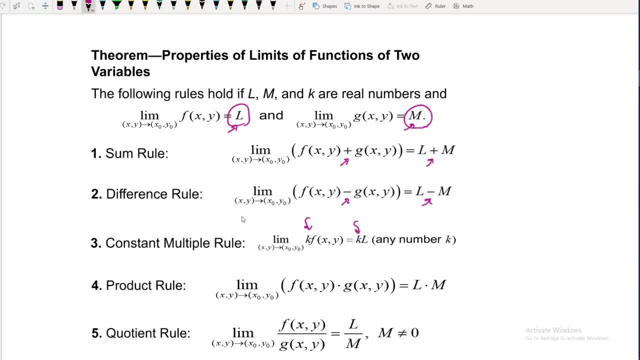 It is equal to k times limit of f of x- y, based on what we had here on this part, It is l, so multiplied by f. So this k is any number. Number four: product rule Limit as x- y approaches x0, y0 of f of x- y multiplied by g of x- y. 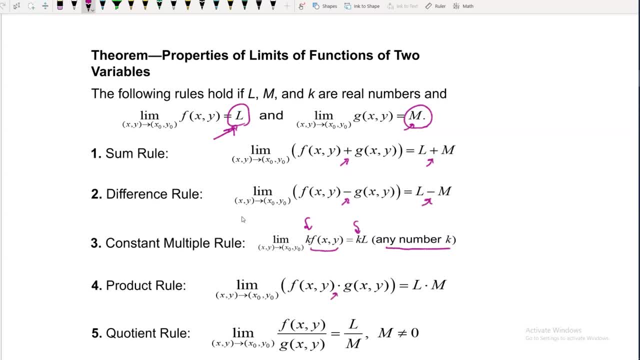 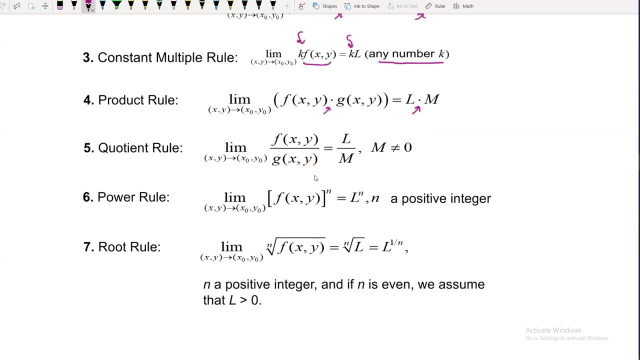 So here we have multiplication. We're going to use again what was given, l and m, but here multiply Number five. quotient rule Limit as x- y approaches x0, y0 of f of x- y divided by g of x- y. 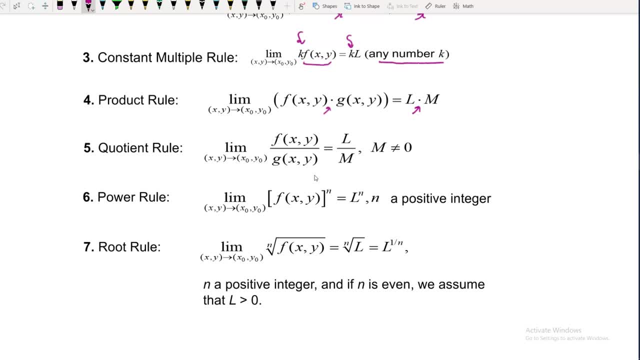 So this k is any number. So this k is any number It is equal to. so here we have division: l divided by m. m is in denominator and denominator shouldn't be equal to zero. So here m is not equal to zero. 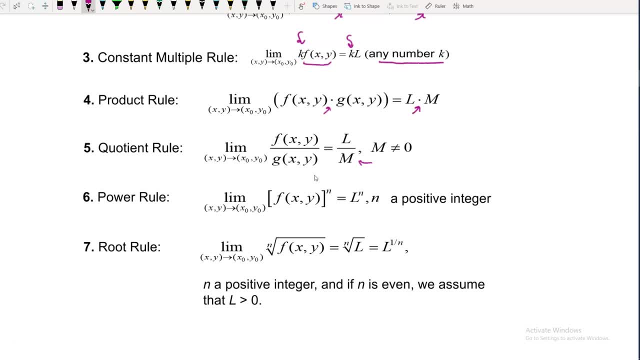 We cannot have zero in denominator. If we have zero in denominator, that means this is undefined. Number six: power rule Limit: as x? y approaches x0, y0 of f of x? y to the nth power, It is equal to. 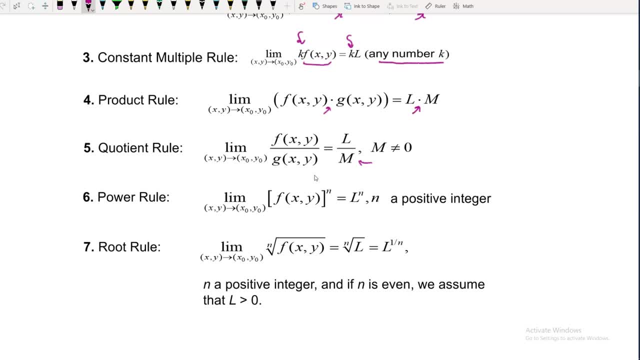 What do we have For limit of f of x? y was equal to l, So use l, and here power It is n. so you have n here as a power and n is a positive integer. Number seven, root rule. 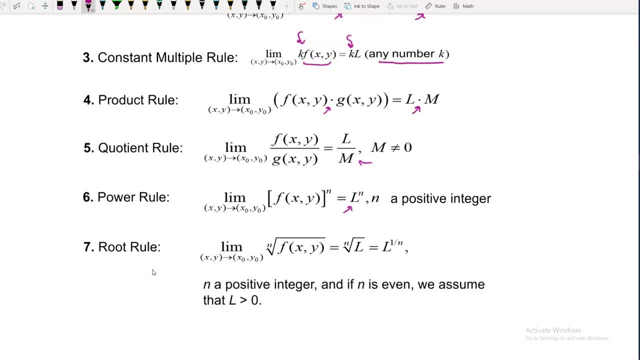 Limit as x y approaches x0, y0 of nth root of f of x y. It is equal to nth root of l, So this is equal to l. power is 1 over n, So n is positive integer and if n is even, we assume that l it is greater than zero. 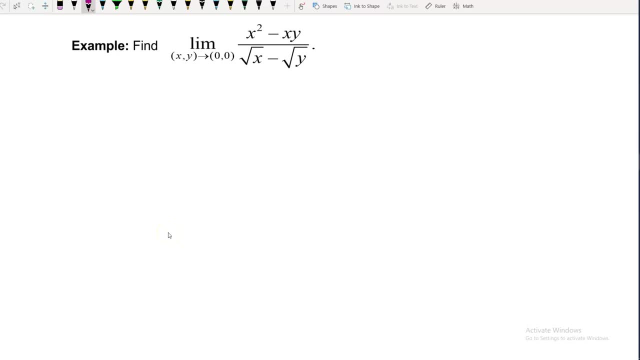 Example: find limit as x. y approaches 0, 0 of x squared minus x y divided by square root of x minus square root of y. If we directly substitute x equal to zero and y equal to zero in this equation, we will have: 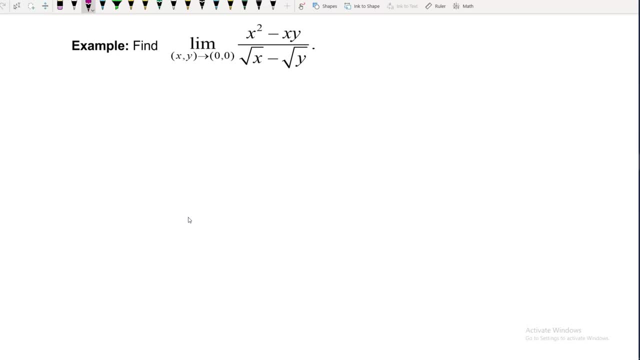 0 minus 0 divided by 0 minus 0. So that will be 0 over 0, and this is indeterminate. And again, because of having zero denominator, we cannot use quotient rule, So I'm going to rewrite what we have here on this part. 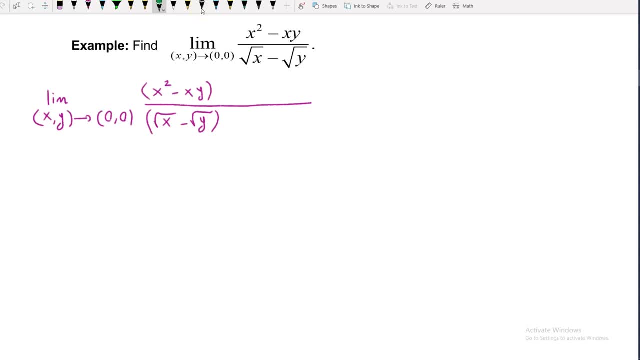 And multiply numerator denominator by square root of x. Here we have subtraction, So here I'm going to use Addition, And this is equal to limit as x, y approaches 0, 0.. So here I multiply what we have in denominator. 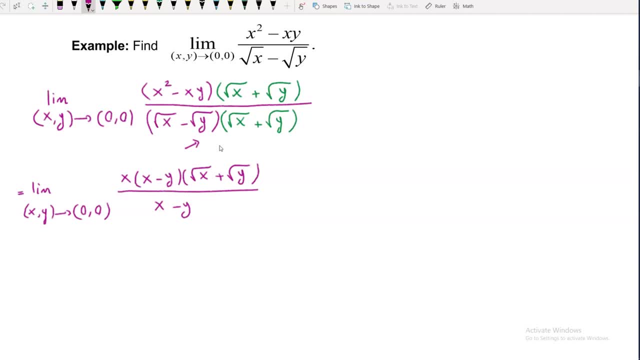 Square root of x times square root of x. Here we have x. Then we have square root of x times square root of y. Negative square root of y times square root of x, So that part is 0.. And finally we have negative square root of y. 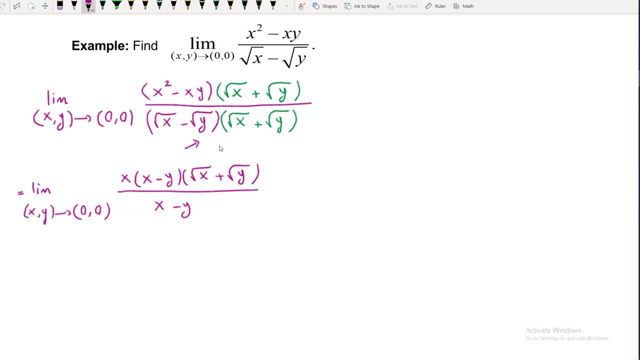 Multiplied by square root of y, So it is equal to negative y. So here we have x minus y in denominator And on top I factor out x. So this part, when we had in common between these two terms, it was x. 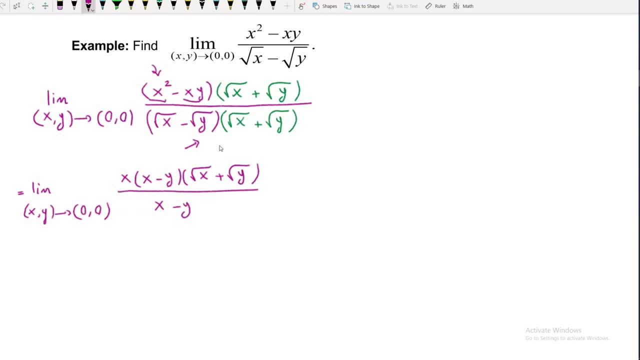 So we factor out x, and that is x times x minus y, And rewrite this part. Now here we can simplify, So we can cancel this part: x minus y divided by x minus y. So here is 1.. Here is 1.. 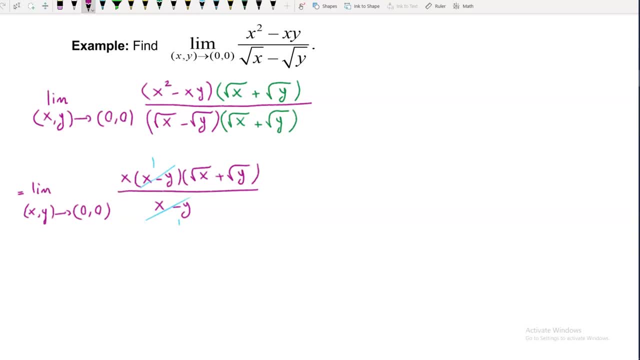 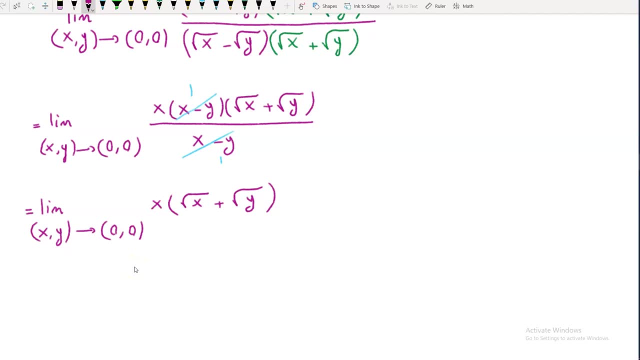 So this is equal to limit as x, y approaches 0, 0 of x times square root of x plus square root of y. Now substitute x equal to 0 and y equal to 0. So here we have 0 times square root of 0 plus square root of 0.. 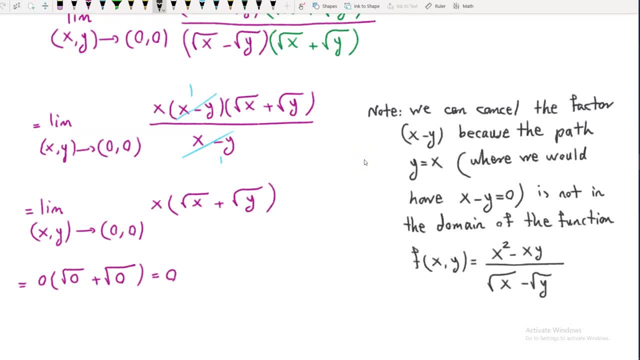 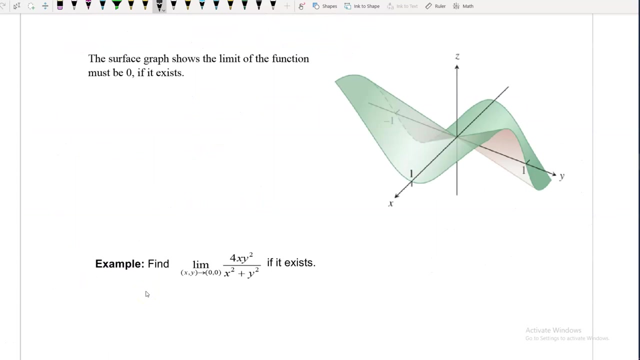 So this is equal to 0.. We were able to cancel factor x minus y, because y equal to x is not, So this is equal to domain of function. So here, on this part, this is our final answer. The surface graph shows that the limit of the function must be 0 if it exists. 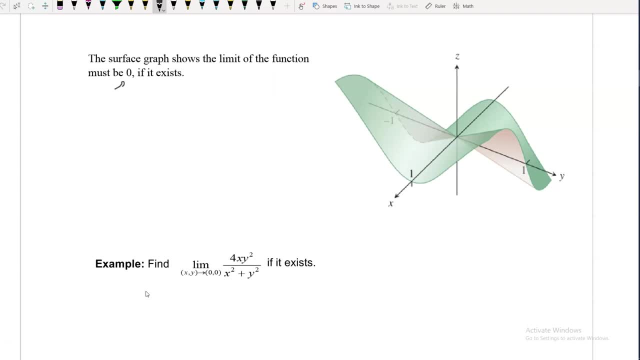 Now here example: find Limit as x. y approaches 0, 0 of 4xy squared divided by x squared plus y squared, if it exists, We first observe that lambda line x is equal to zero. The function always has value zero, So here I substitute zero for x, And this is when y is not equal to zero. 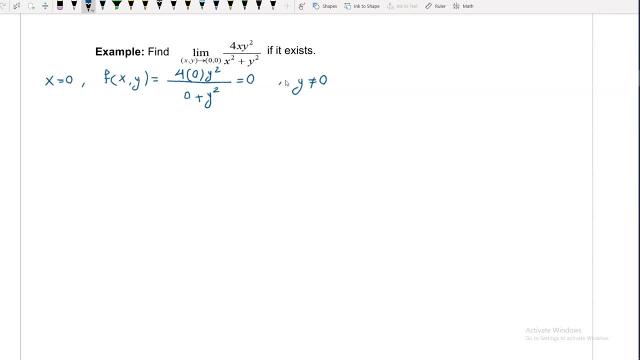 Because here in a denominator we don't want to have zero And along to the line y equal to zero, the function has value zero when x is not equal to zero. So if the limitless exists as x, y approaches lambda Point, The value of limit must be zero. 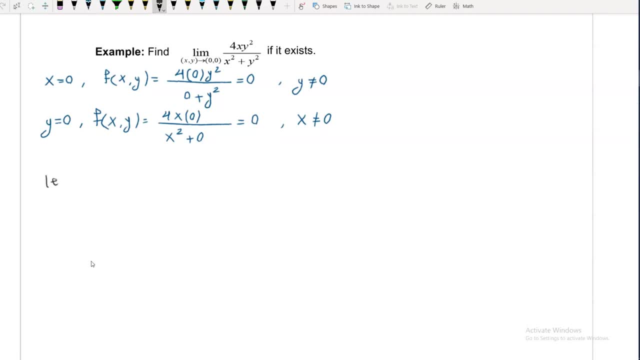 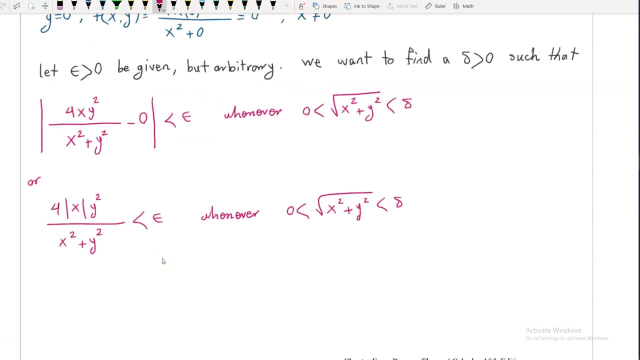 Let epsilon greater than zero. We want to find delta greater than zero, such that absolute value of 4xy squared divided by x squared plus y squared minus zero, less than epsilon, whatever Square root of x squared plus y squared between zero delta. 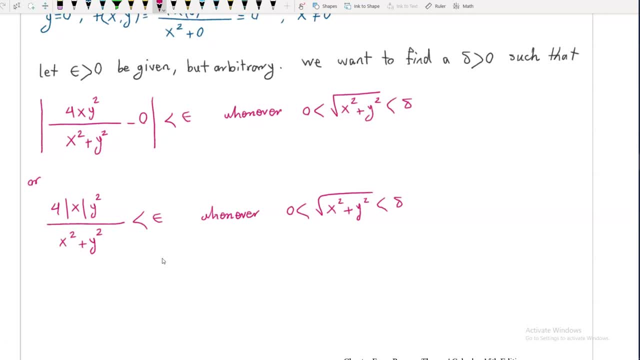 All. Since y squared is less than or equal to x squared plus y squared. Since y squared is less than or equal to x squared plus y squared For times. Absolute value of x times y squared divided by x square plus y squared, Which 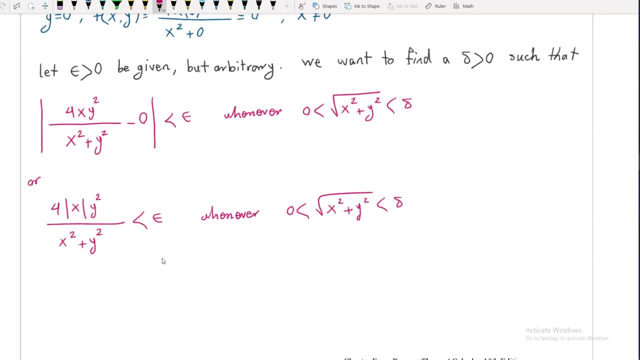 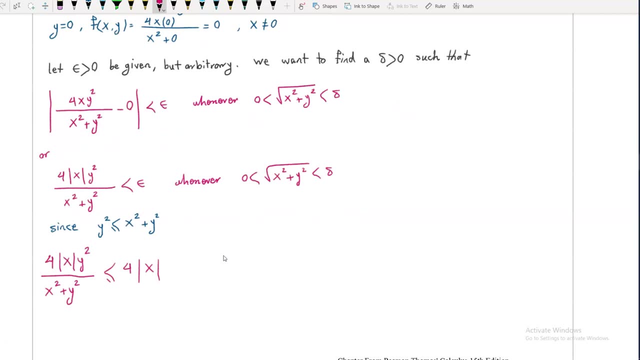 When the rule Engineering uses the baton's being the sun. Noout of this comes down to: x is equal to, As if I change from x times at the bottom of X. So based on what we had here on the score, we have y squared less than or equal to x squared plus y squared. 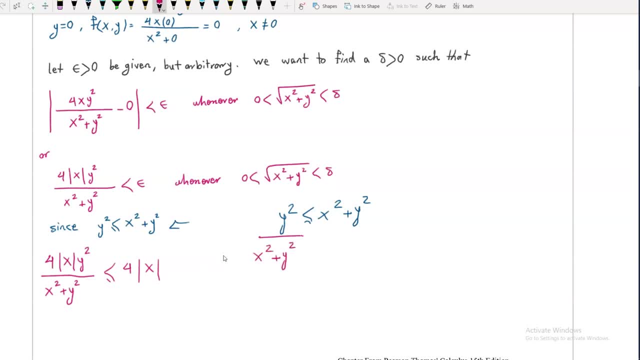 If I divide by x squared plus y squared, both sides, this part cancels. So here we have y squared divided by x squared plus y squared, It is less than or equal to 1.. So use this part, which is here: 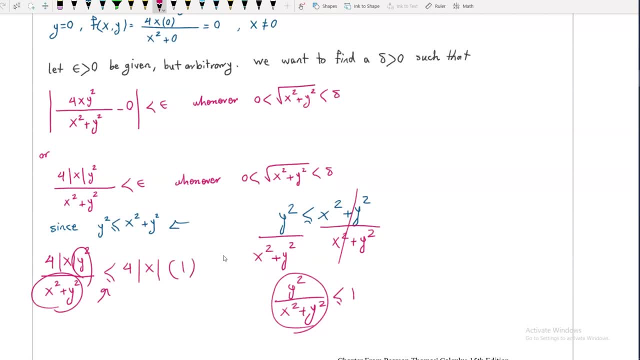 And that part is less than or equal to what we have here, less than or equal to 1.. I'm going to erase this part And then next step from here. this is equal to 4 times. Instead of absolute value of x, I can use square root of. 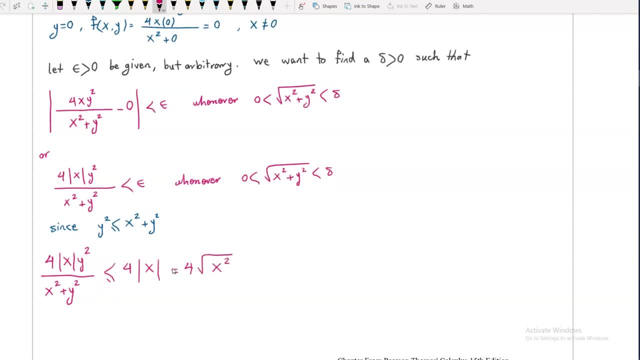 So x squared and this is less than or equal to 4 times square root of Here again we can use x squared less than or equal to x squared plus y squared. So this is the same as what I did on the first part. 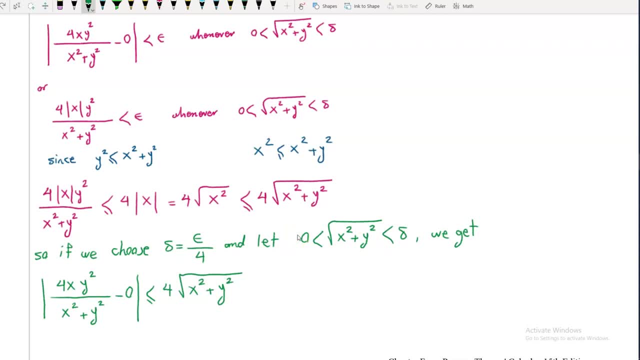 So if we choose Delta equal to epsilon divided by 4, and let square root of x squared plus y squared between 0 and delta, Here we have absolute value of 4 x y squared divided by x squared plus y squared minus 0,. based on what we have here, 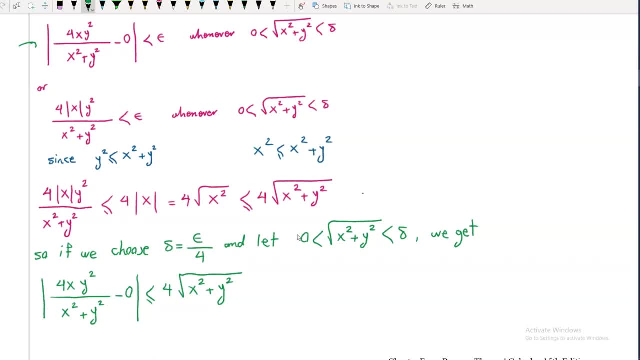 And that one was less than or equal to what we had here on the score, And that's 4 times square root of x squared plus y squared. And then This is less than or equal to 4 times. using what we have here, square root of x squared plus y squared is less than or equal to delta. 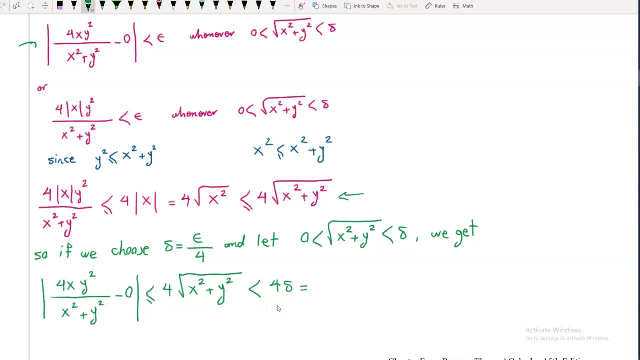 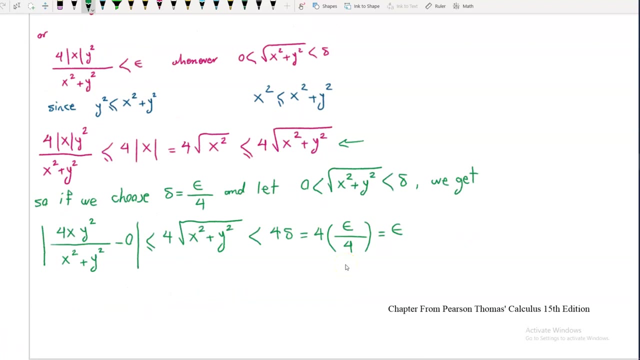 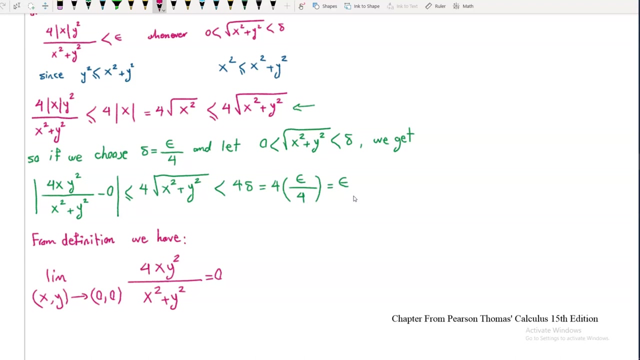 So here we have 4 times delta, and that is equal to 4 times based on what we have here, And that is 4 times epsilon divided by 4. And this is equal to epsilon. So this means absolute value of 4 x- y squared divided by x squared plus y squared, it is less than or equal to epsilon. 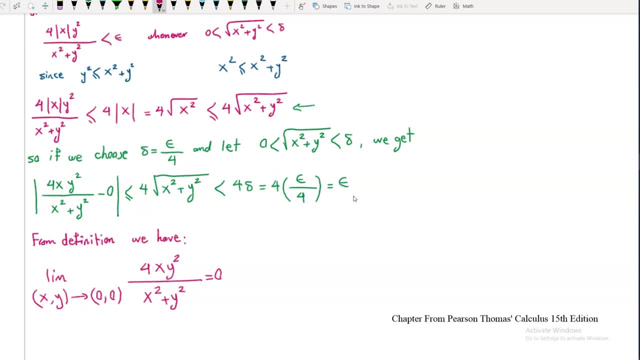 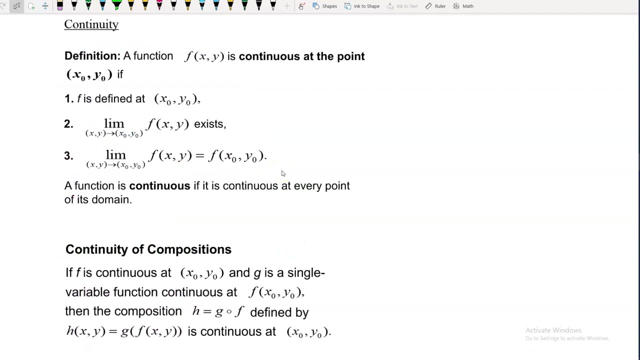 And from definition we have limit as x- y approaches 0, 0 of this function: 4 x- y squared. divided by x squared plus y squared, it is equal to 0.. Definition of function f of x- y is continuous and defined. 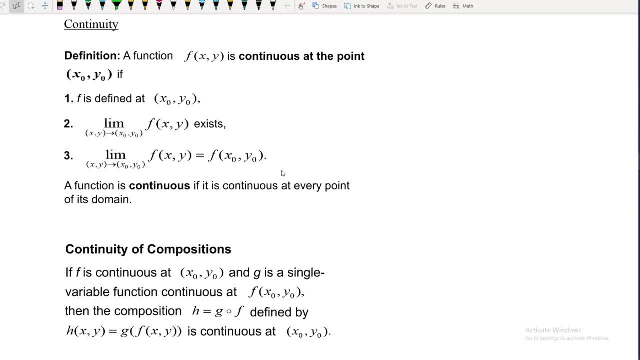 We only have default of point x, naught, y, naught. If f is defined at this point, x, naught, y naught limit. as x- y approaches this point of f of x, y exist limit. as x- y approaches this point of f of x- y, it is equal to f of x, naught, y naught. 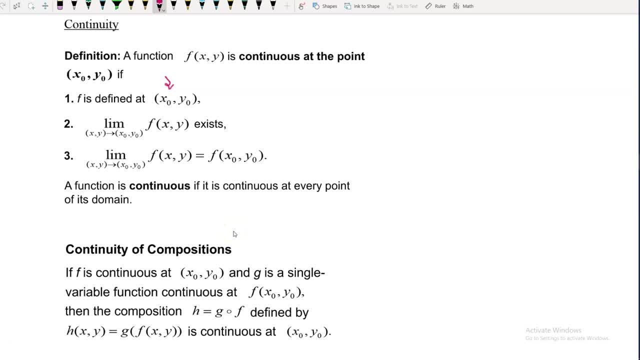 Function is continuous at every point at this point, every point of its domain. continuity of compositions. if f is continuous at this point, x naught, y naught and g is a single variable function continuous at f of x, naught, y naught, then composition h. it is equal to g of f, defined by h of x, y and is equal to g of f of x, y is. 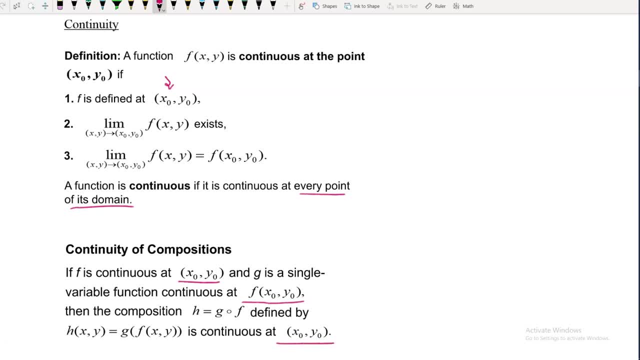 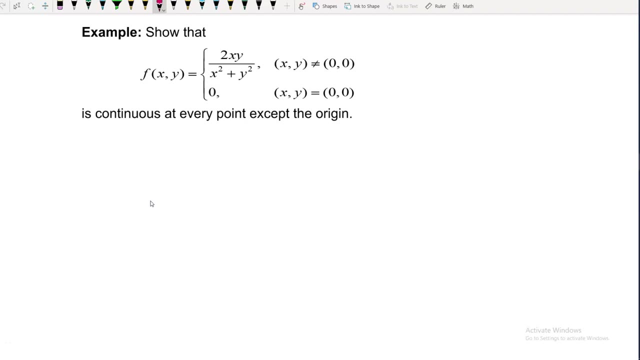 continuous at this point x naught, y naught. so in this part here f, it is inner function and g is outer function. show that f of x, y equal to 2, x, y divided by x square plus y squared, and the point x, y is not the origin. so here we have x, y is not equal to 0, 0 and f of x- y. 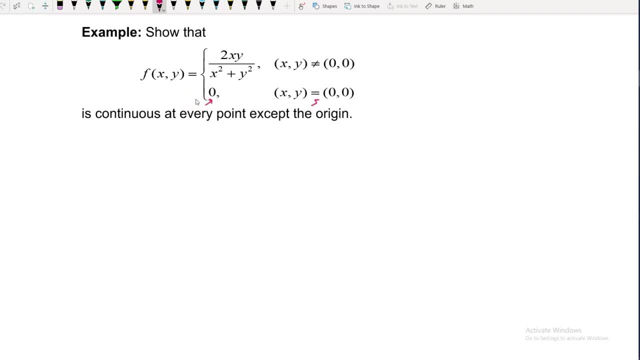 equal to 0 and at this point origin, so x, y, it is equal to 0. 0 is continuous at every point except the origin. so when the point x, y is not the origin, so it's not equal to 0, 0, this function is defined at every point. so to show that the function is not continuous at the origin. 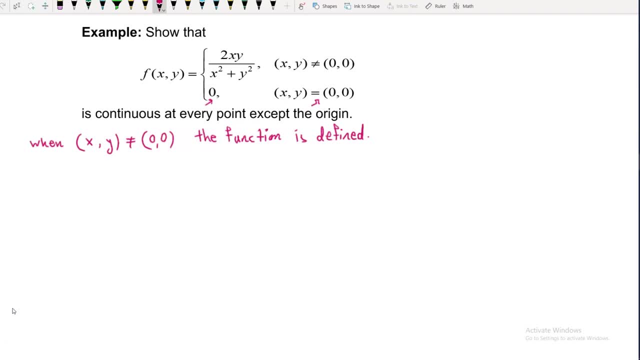 we. we need to shut out the limit as x0 approaches 0, 0 of our function f of xy, f, f, x, o does not exist. we are going to approach the original among the lines of the forward angle: y equal to normal, ут painful to m. 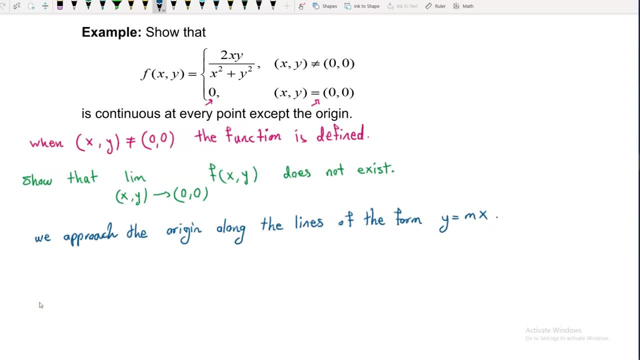 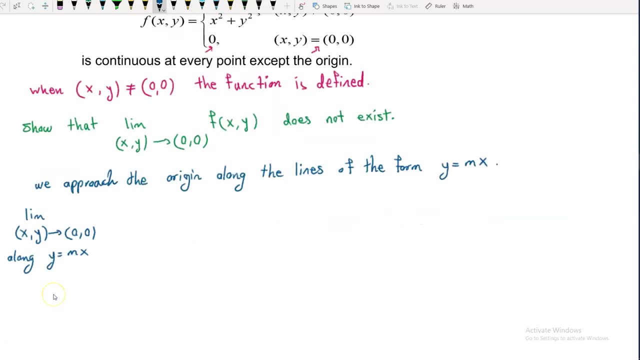 because if the expressed at the origin, you must get the same value for the limit. now other opaque curve of the curve sala, we approach the original line Kaleega to evaluate the limit as xy approaches 0,, 0 along y equal to mx of a function f of xy. 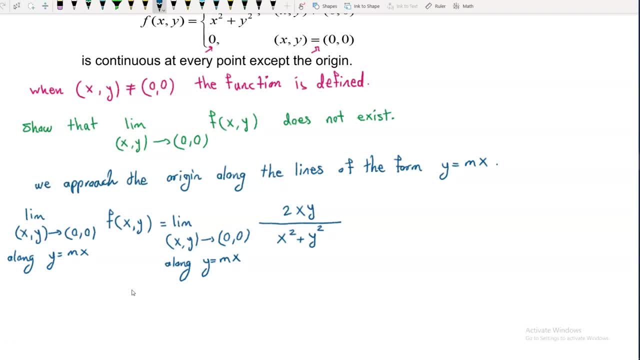 So this is equal to the limit as xy approaches 0, 0 along y equal to mx of this function to xy over x squared plus y squared. So now substitute y equal to mx here in this function, So this is equal to 2x instead of y. 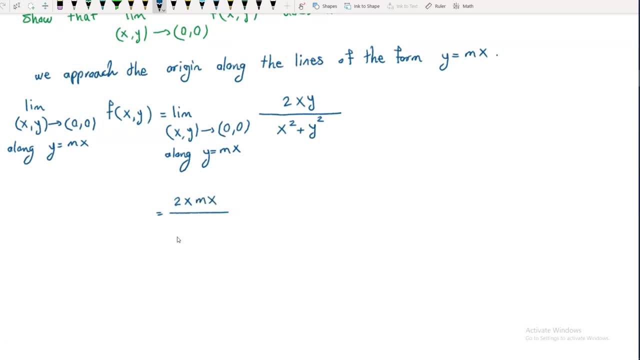 Now here we have mx divided by x squared plus mx squared, And this is equal to 2mx squared over x squared plus mx squared. So this is equal to 2mx squared over x squared. And now this is equal to 2mx squared. 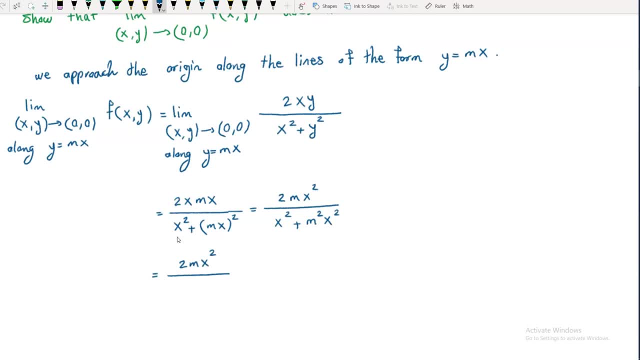 Now here we have common factor. it is x squared, So x squared times the factor and we have 1 plus m squared. This is equal to- we can simplify, so cancel. So x squared here is 2m over 1 plus m squared. 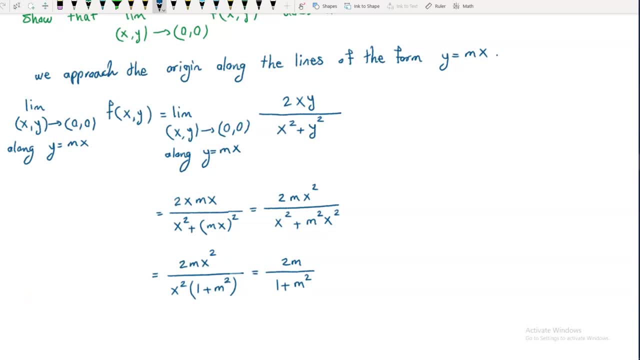 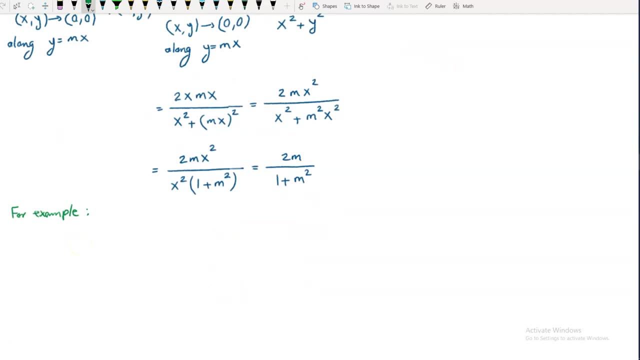 If we substitute different values for m, we're going to have different values for the limit. For example, if m equal to 0, limit as xy approaches 0, 0 of f of xy is equal to 2 times, So that's instead of m. now here we have 0. 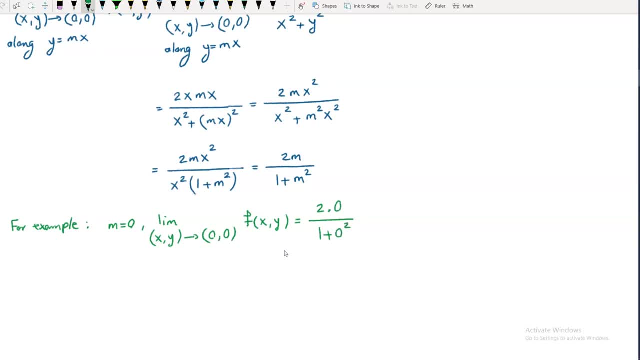 So this is equal to 1.. So this is equal to 0.. And if m equal to 1, limit as x minus 0, 0 of f of xy is equal to 2 times 1 divided by 1 plus 1 squared. 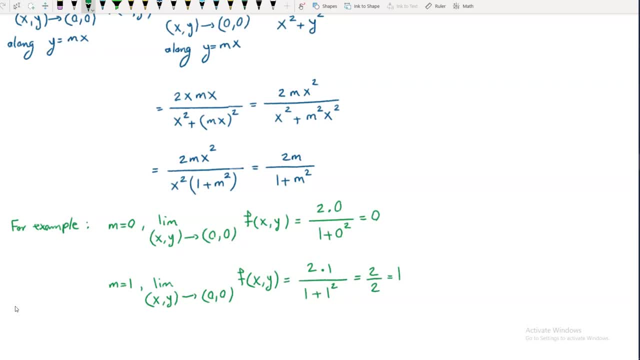 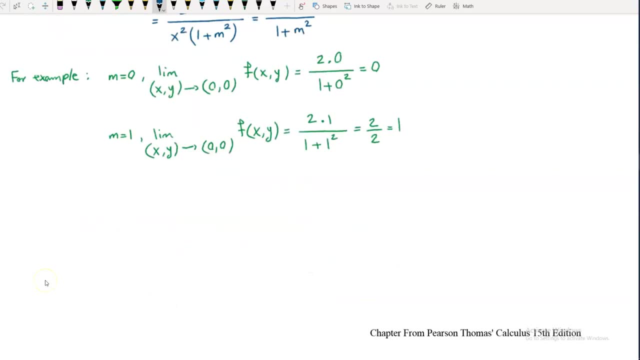 So this is equal to 1.. This means for different values of m, we get different values for the limit. So, by definition, limit does not exist. So as the limit changes with each value of the slope m, the long-based one that we have here for y equal to mx, m is the slope. 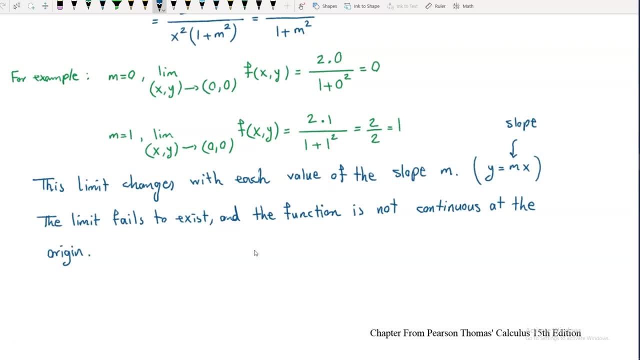 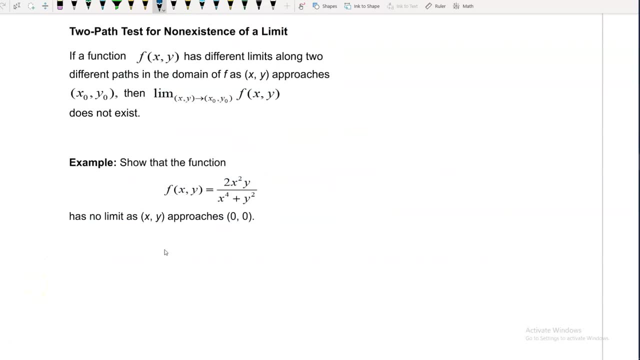 the limit fails to exist and the function is non-continuous at the origin. To pass tests for non-existence of a limit, if a function f of xy has 0, 0 of f of xy, limits belong to different paths in the domain of f. as xy approaches x0, y0, then 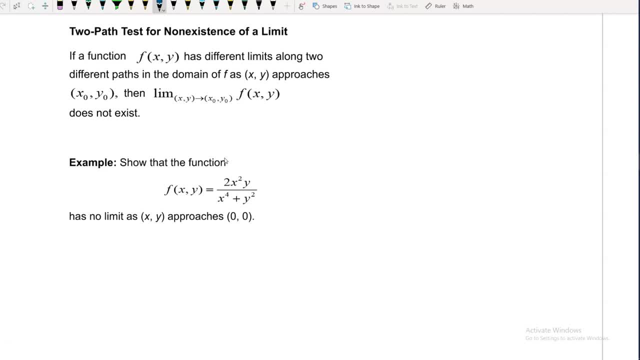 limit as xy approaches x0, y0 of f of xy does not exist. example show that the function f of xy, which is equal to 2x square, y over x to the fourth power plus y square, has no limit as xy approaches origin. 0 comma 0. so if the limit 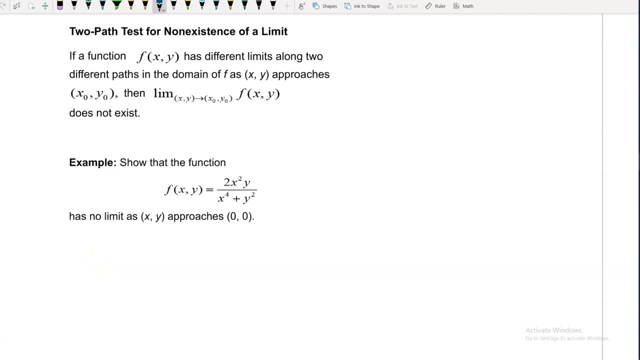 exists, we would have to show that at the point x, y approaches the origin. along any curve we must get the same limit value. but here, in this case, limit does not exist. let's find two curves that as we approach the region we end up having different limits. so first let's look at the